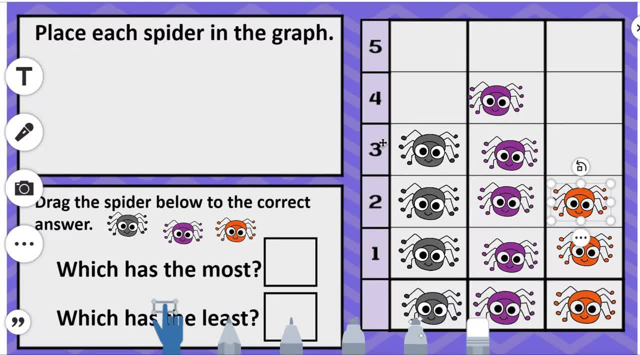 ends here at this number. that number is three, so that means that I have three black spiders. now, remember, we can't count this one here, nor this one or this one, because these are our labels. this is: these are the pictures that tell us where to put our spiders. so we don't count these down here. so, because it ends. 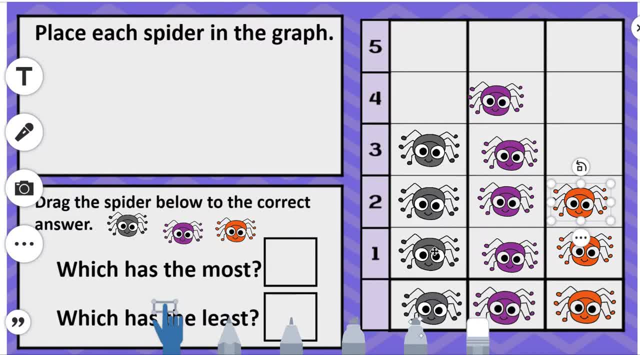 here, then I can very clearly see that I've got three black spiders. but look at the purple one. the purple one, look how tall it is. and it ends here. so that number is four. I don't even have to count the spiders. if I don't want to, I can just come over. 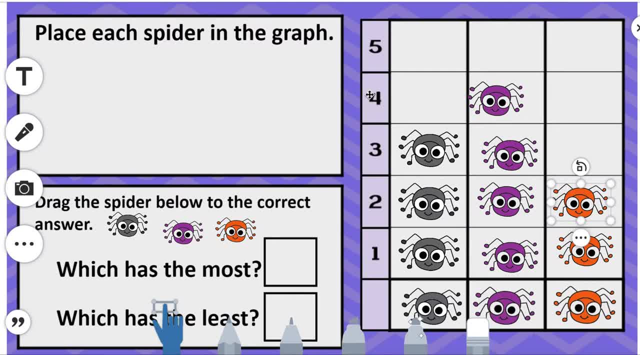 here and look at the number here on the left-hand side of the bar graph and I can clearly read that there are four purple spiders and then finally the orange. I just come over here across, see that, see where the last one is, right here I go across and I can see that I only have two. I can check it if I want. 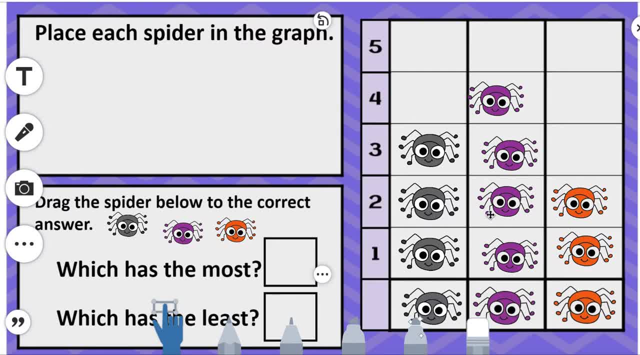 to two, and I would be correct. so we've already created our pictograph. now we're going to analyze our data. that means we're going to take a look at it and then we're going to draw conclusions, which means we're going to be answering some questions. so our question here is: which has the most? hmm, do we have more? 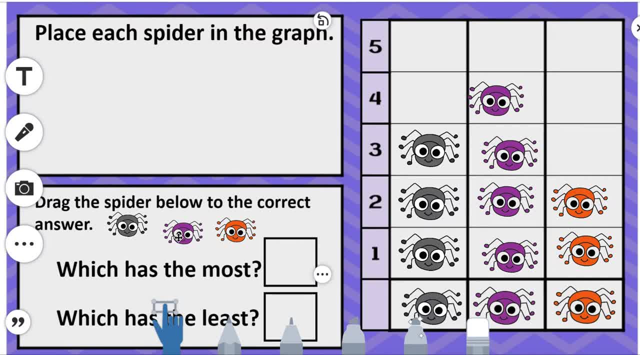 black spiders, purple spiders or orange spiders? well, let's take a look at the graph. I see we've got three black spiders, four purple spiders and two orange spiders. which one do you think we have the most of? that's right. purple, yes, because look how tall it is, but also you can see that the number is four and four. 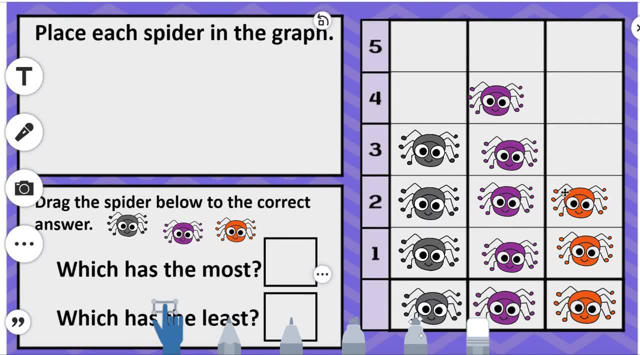 is more than three and four is more than two. so I'm going to take a look at the graph and I'm going to take a look at the number of spiders. so I'm going to come over here, click on my purple spider and place them in the box, and then the last question is: which has the least? so which? 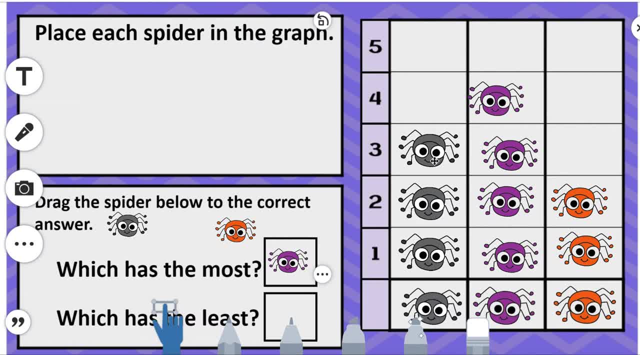 one did we have the least of? hmm well, I can see that the black spiders, those are less than the purple. but when I look at the orange spiders I can see that the There's less orange spiders than purple spiders And there's definitely less orange spiders than black spiders. 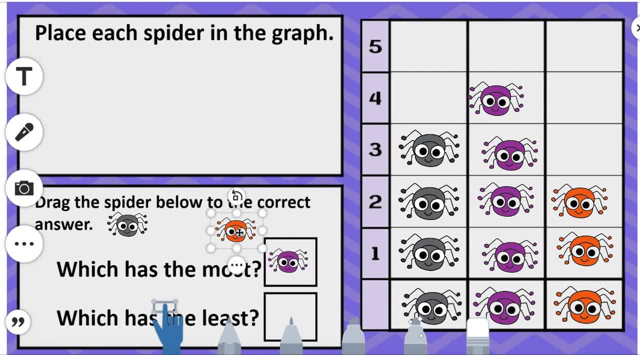 So I think that the orange spiders is the one that we have the least of All. right boys and girls. and I'm finished. I'm going to click my green checkmark to submit my work. And good luck, because you're going to do the same thing. Thank you. 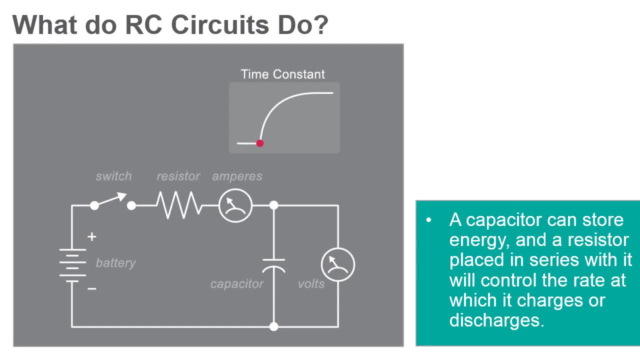 A capacitor can store energy and a resistor placed in series with it will control the rate at which it charges or discharges. This produces a characteristic time dependence that turns out to be exponential. The crucial parameter that describes the time dependence is the time constant also. 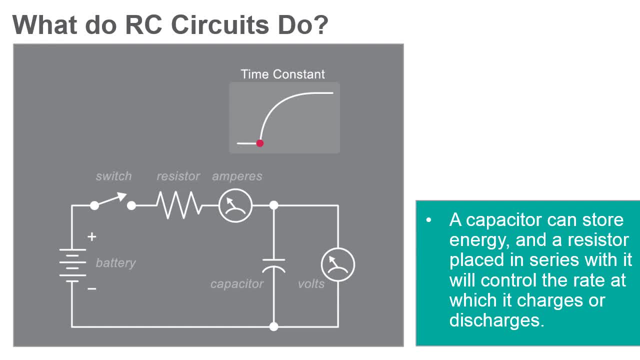 called tau RC For RC circuits. tau is simply equal to R times C. The simplest RC circuit is a capacitor and resistor in series. When a circuit consists of only a charged capacitor and a resistor, the capacitor will discharge its stored energy through the resistor. When a circuit consists of a power supply, a 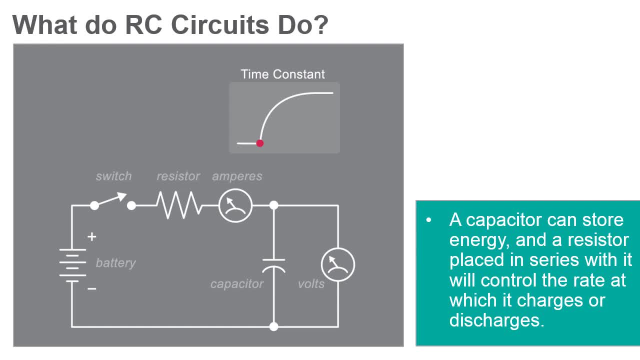 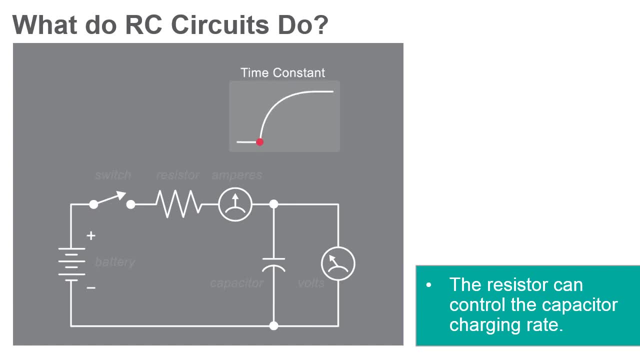 resistor and an uncharged capacitor. the capacitor will charge based on the current flowing through the resistor. The resistor is often used to control the rate at which the capacitor charges and discharges. Time constants in RC circuits can sound intimidating, but they are not. 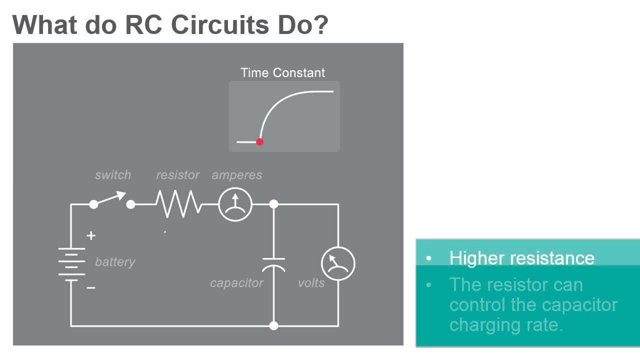 But the behavior is relatively simple when you think about it. With a higher resistance, the current in the circuit is decreased and the capacitor charges more slowly. With a lower resistance, the current in the circuit is increased and the capacitor charges more quickly. RC circuits can be used to filter a signal.